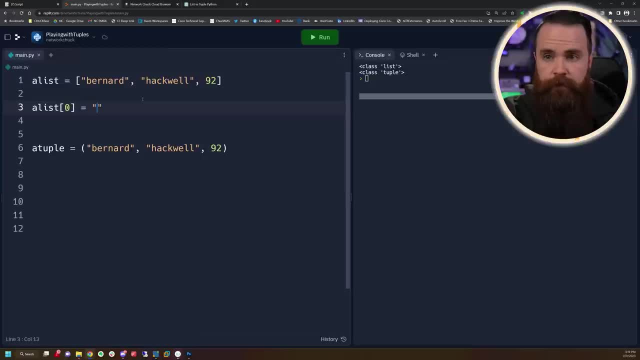 We'll change Bernard to Chuck. We'll say index zero equals Chuck And we'll print that list to see what it looks like. Nailed it. It changed mutable. Let's try to change our tuple- Same process called the zero Index- and have that equal Chuck And we'll try to print it out. 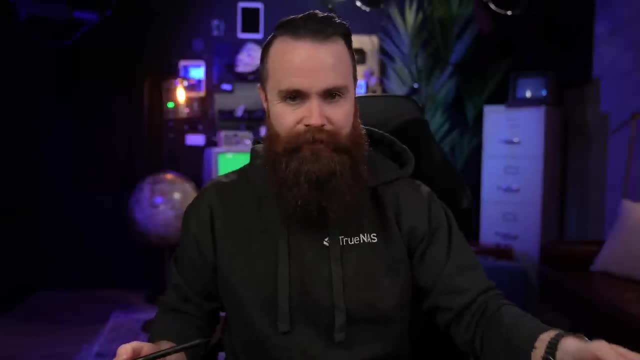 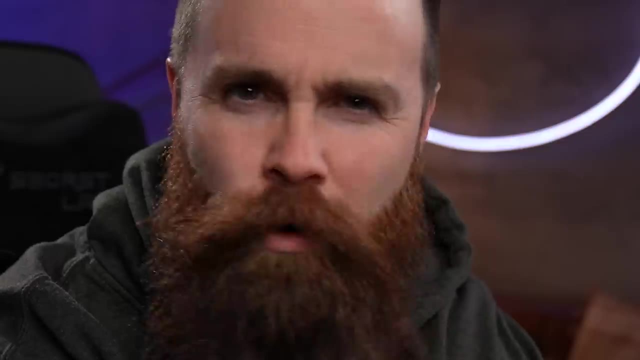 Can't do it. It's immutable, Can't touch this. Sorry, I had to do it So we could stuff their video over case closed. But if you're like me, you might be wondering: so what? So what if you can't change it? I still don't see the reason. the use case. 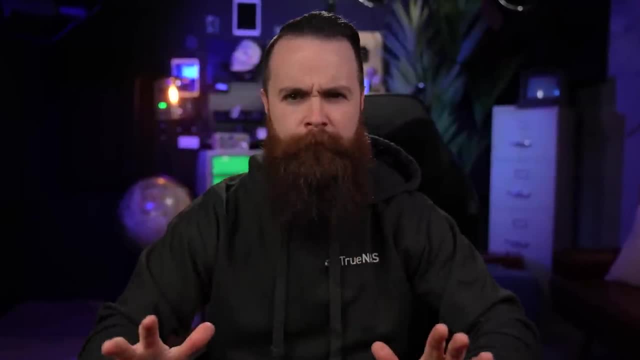 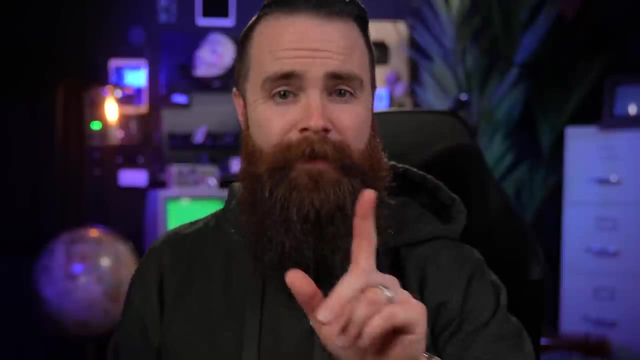 because it still seems like we're trying to overcomplicate something That should be very simple. Just make it a list. The list does everything. So I dove deeper, or real quick. before we overcomplicate things with tuples and lists, Let me tell you something That's not complicated. 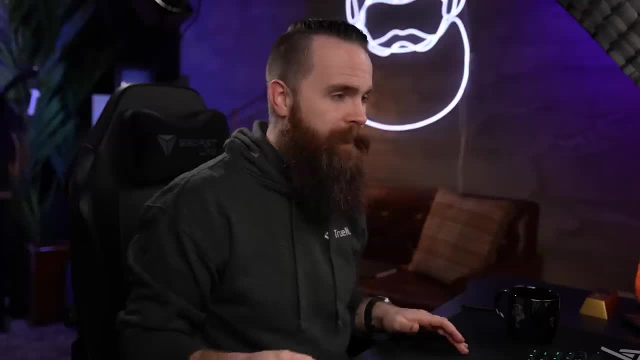 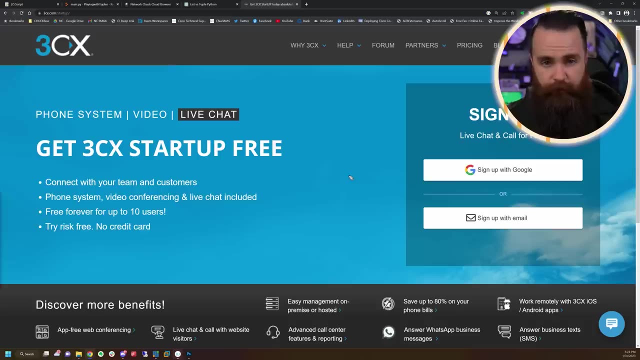 After this video: three CX. three CX is something you want to play with because having you always wanted your own phone system, Yes, you have. you're about to get one for free. Three CX has a new thing. It's called three CX startup, Now in the full system world. 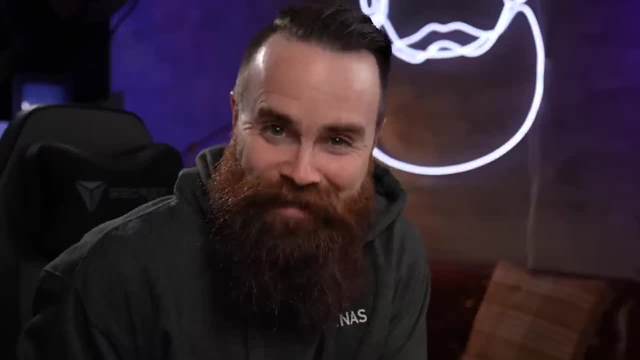 things can get pretty complex, Like it was my whole job. That's how much of a pain it was. But here you get the whole shebang: live chat, video chat, a phone system And it's in the cloud like legit. 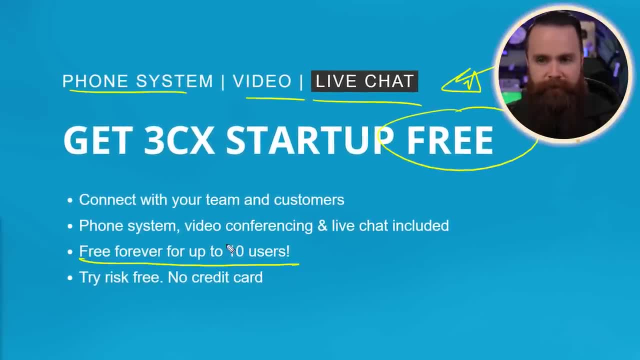 they're doing this And I don't know how they can do this, but it's free forever for up to 10 users. Like seriously, just try this out. It's really fun putting your own phone system right now. Take it five minutes. 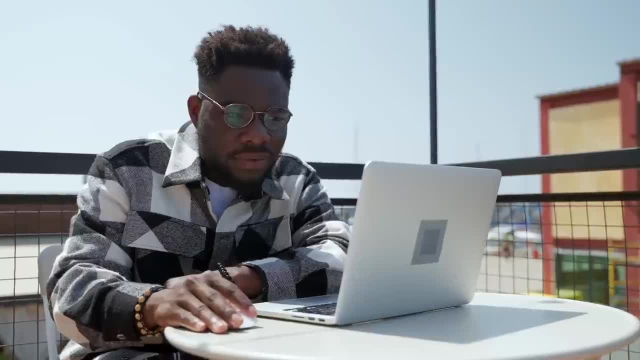 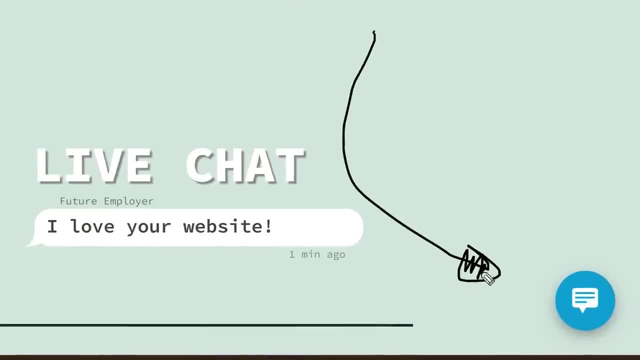 Nothing Makes me feel more professional, More professional than having live chat on your website. Let's say you're a person in it and you want to have a killer resume portfolio website. Imagine if you had live chat on there and a recruiter could come on your website. 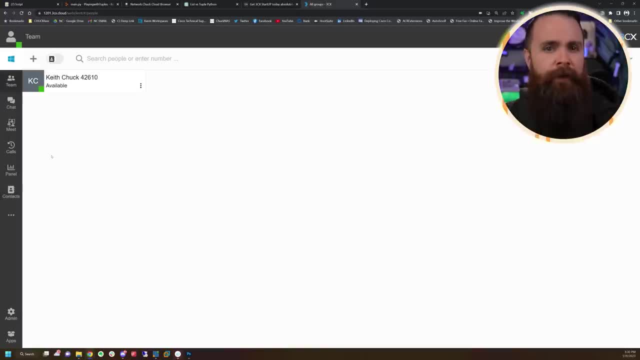 and just start chatting with you. I did this just now. Now, it took me about five minutes to set up my cloud phone system. That's kind of stupid easy, And then adding my live chat to WordPress took just a few moments. Check it out. 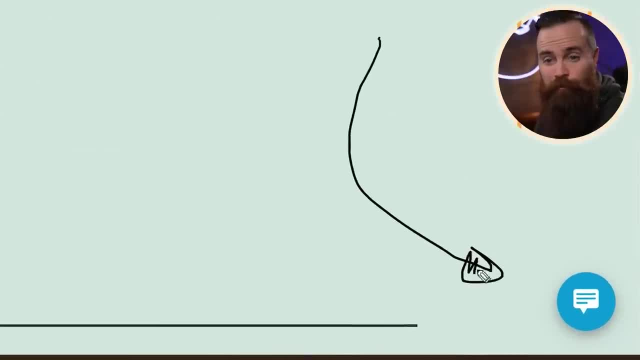 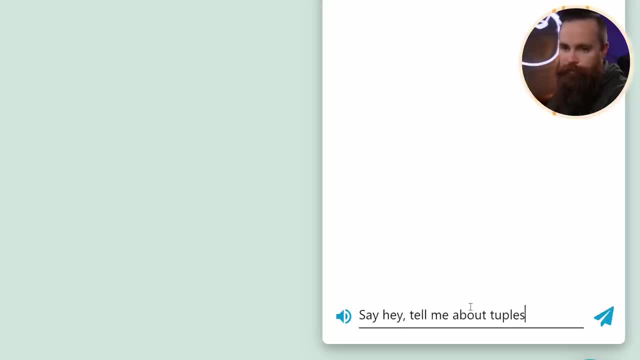 Do you see that at the bottom right chat icon? because they have a WordPress plugin and it took no time at all. I keep saying that, but that's literally what it took. Say, Hey, tell me about two. and then bam, looking back at my three CX web client, there's the chat right there. 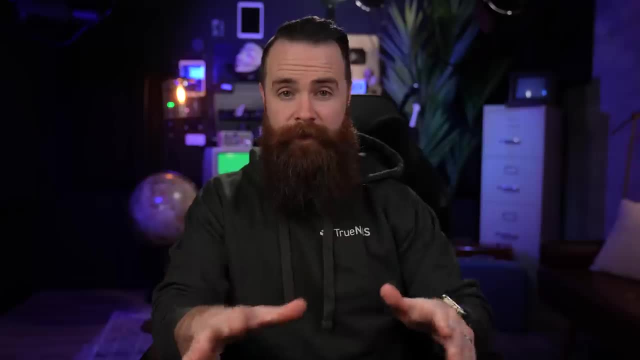 Two pools are stupid And I'm helping my client learn about two pools. They don't only have a web client, They've got a client for your phone- Android and iOS. They've got a desktop client. It's stupid How awesome this is. 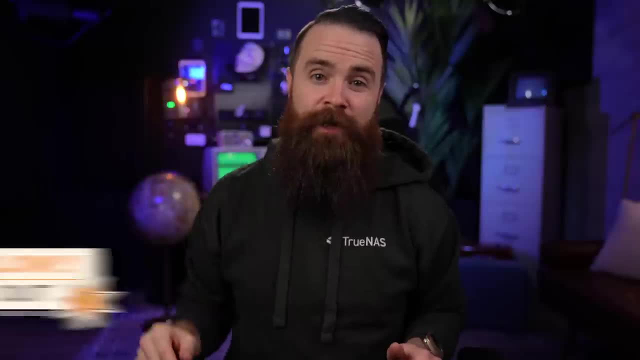 And it's kind of crazy that they're giving it away for free for up to 10 users. Check it out below. Anyways, back to tools and how stupid they are. I'm just kidding, They're actually pretty cool. That's what I learned. 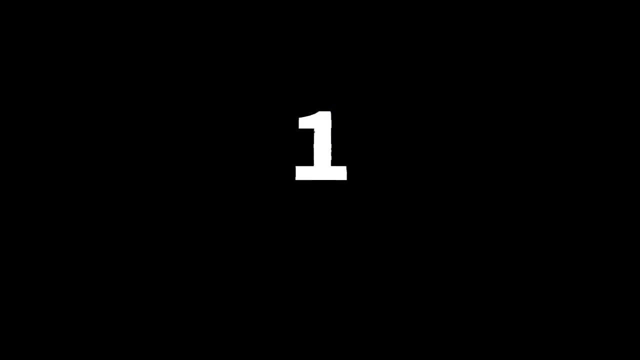 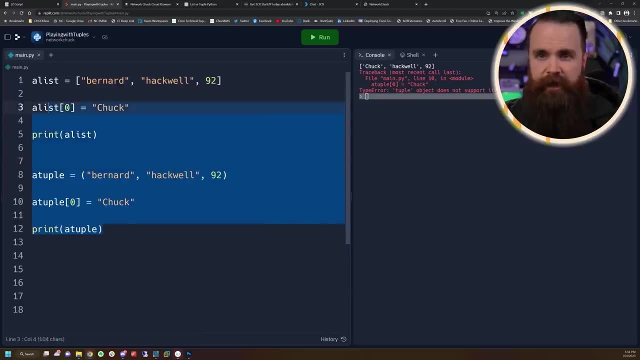 I asked Google again and I asked my discord, and here's what I learned: Two things. Number one: the fact that two pools are mutable means they're faster than lists Like. let me show you demonstration time using a tool called time it. We're going to see how fast Python can create. 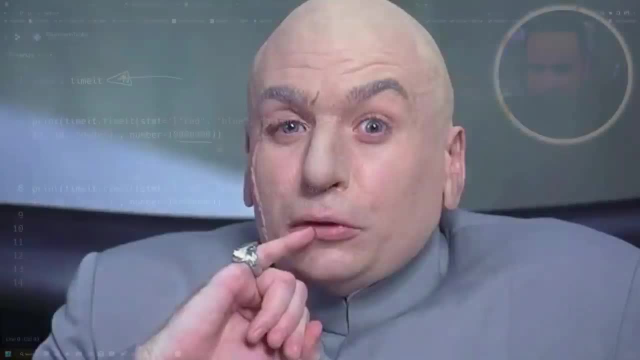 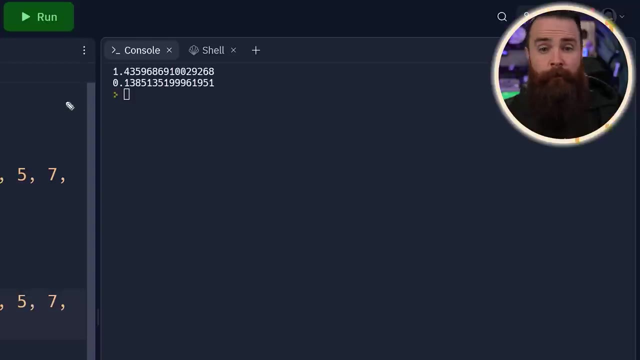 How many, did I say? How many zeros are here? 1 million lists and 1 million tuples Ready, Set go. The results are in and it's obvious: 1.43 seconds for a list and 0.13 seconds for a tuple. Dude that made a list cry. 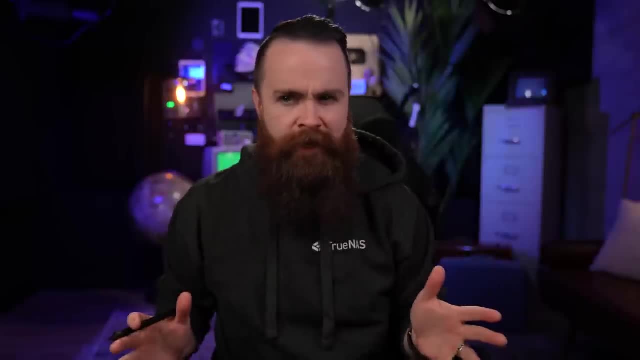 But now I'm sure you're wondering: why is a tuple faster than a list? They're doing the same thing, right? No, And it's back to mutability, Our favorite word- And it has to do a storage, because a list is mutable. 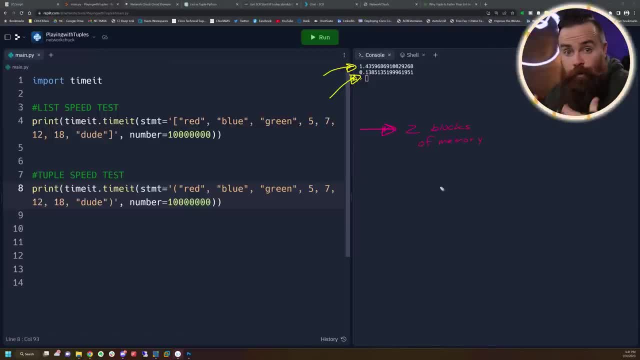 You can change it. It's stored in two blocks of memory to allow for new data, change data, Whereas a tuple it's stored in one block of memory. It's not going to change. And now I know, in our example, this little millisecond difference in time. 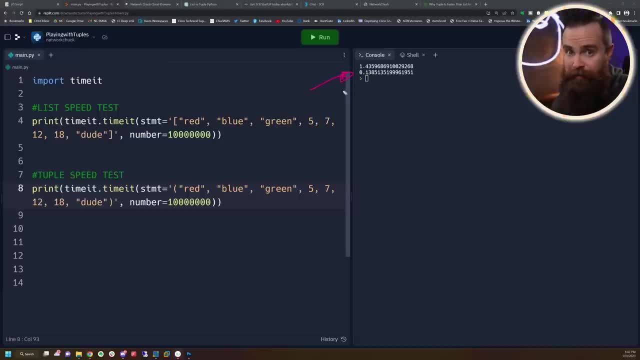 it doesn't seem like a big thing, but in large bulky programs I could be time, save money. say so okay. At this point I'm kind of convinced I get it. Two pools are pretty cool. They're fast and I like fast. 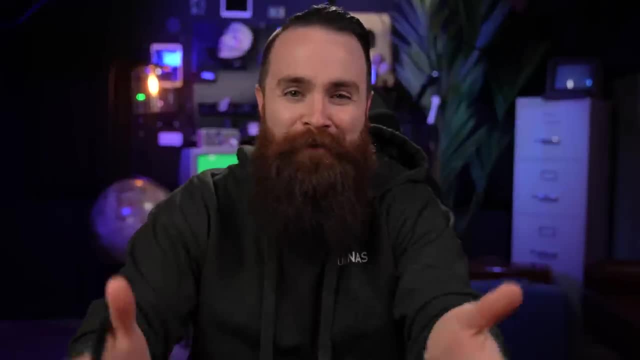 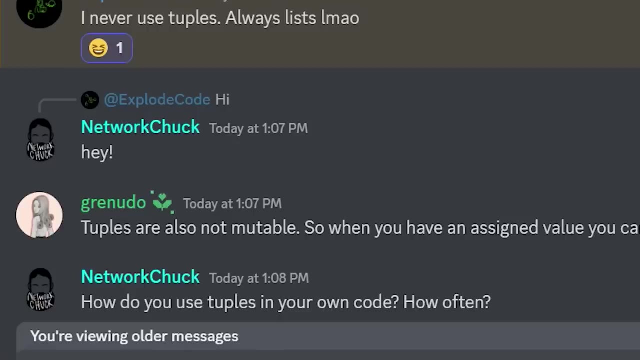 but now on to point two, as to why we use two pools, and that's: why do we use Two pools? What's the use case? When am I going to need data that can be changed? And for that I asked Google and my discord, and I got fantastic answers. 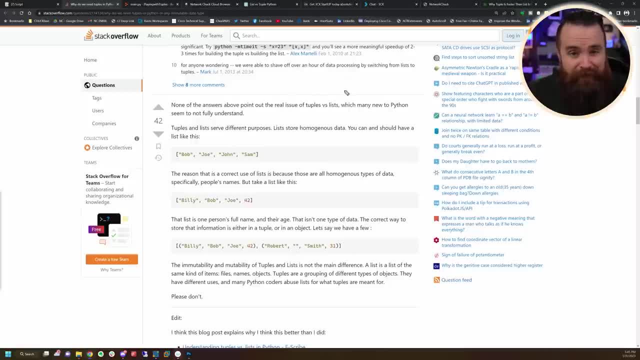 I found a really great answer on stack overflow and it has to do with the types of data you might want to store in a list. versus a two and a list, You'll want to store what's called homogenous data. It's just kind of fun to say. 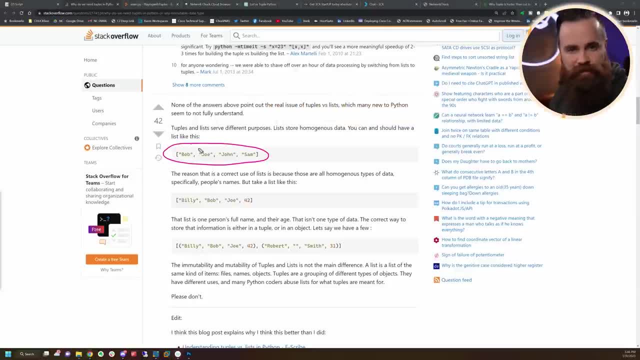 go ahead and say homogenous. For example, a list of names all strings the same type of data: list of coffees, list of YouTubers. These are examples of data within a list that we might add, to change, remove. 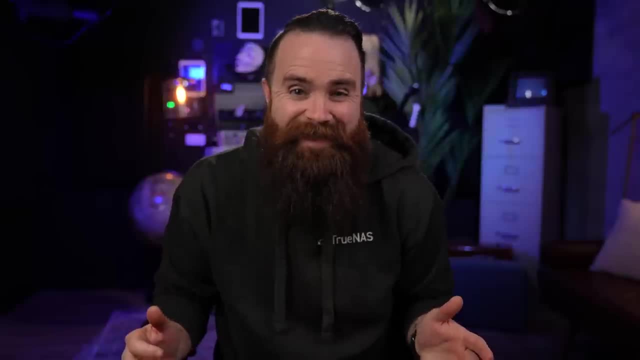 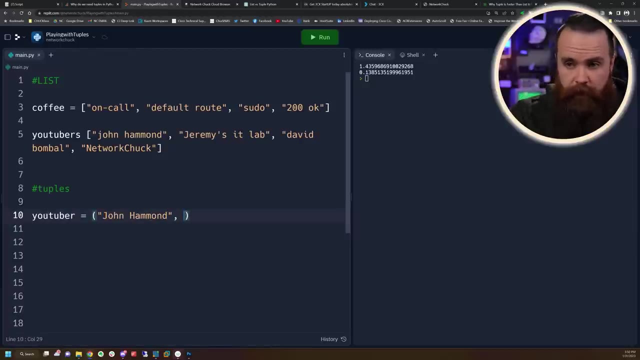 but in two pools. you might use hair header header in this data. I can't say that, So I might have one two pool called YouTuber and it would contain data about a YouTube name subscriber count. How many has John Hammond have now? Ooh, 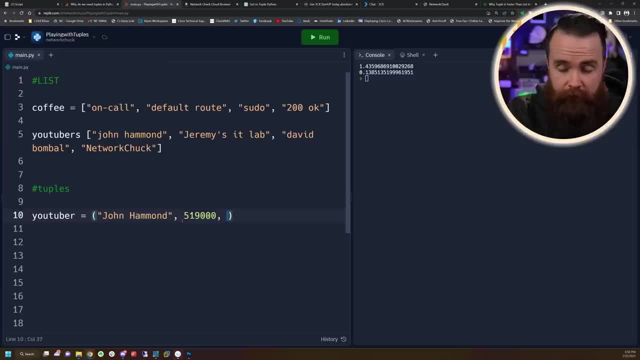 519,000 way to go John Hammond and the types of videos He makes, packing heterogeneous data. Did I say it right The first time or second time? that felt really good. It's all different, but it's all data pertaining to a certain YouTube business. 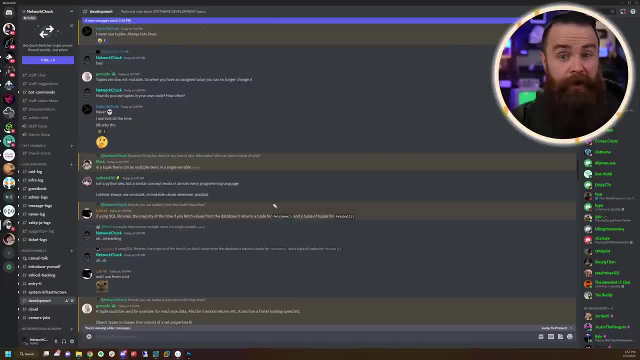 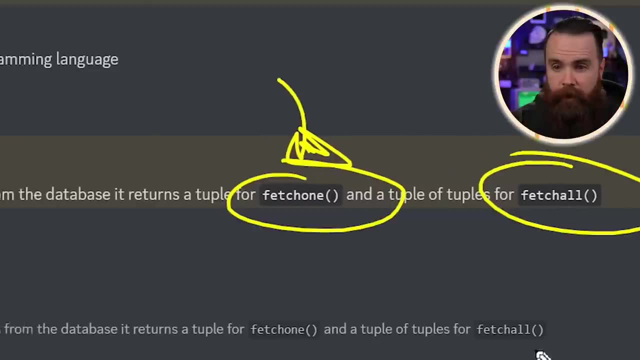 How we're grouping our different types of data And when you're working with SQL libraries and Python, you're actually kind of forced to use tuples. They often return tuples When you use things like fetch one, fetch all and similar methods. I think you will have Brett in my discord And, by the way, 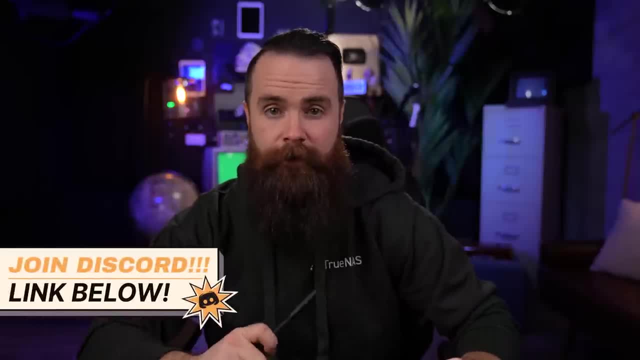 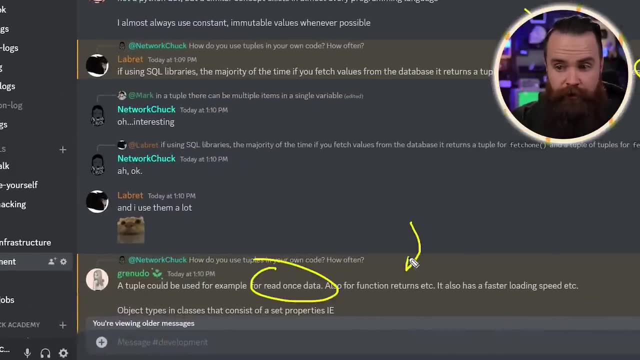 if you haven't joined my discord, check it out. Super helpful, amazing people in there That'll help you on your Python learning journey. And Granito also points out that you want to use a tuple for kind of read. once data, quick stuff and function returns for faster loading speed. 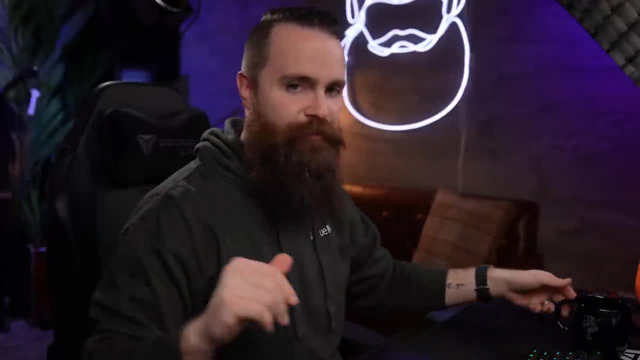 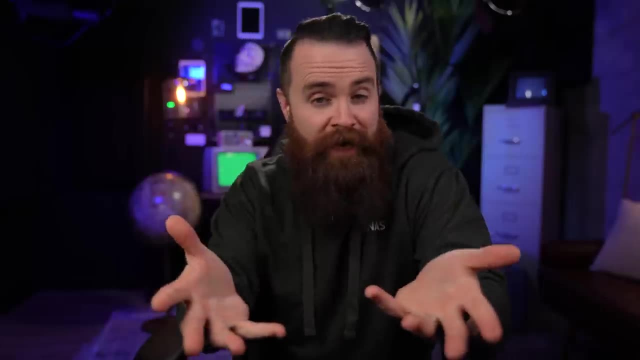 We'll talk more about functions later. It's okay, I get it. Two pools have their place. They're a thing I might start using them- Probably not, but they're also kind of weird. Let me show you some weird things you can do with. actually, this one's kind of 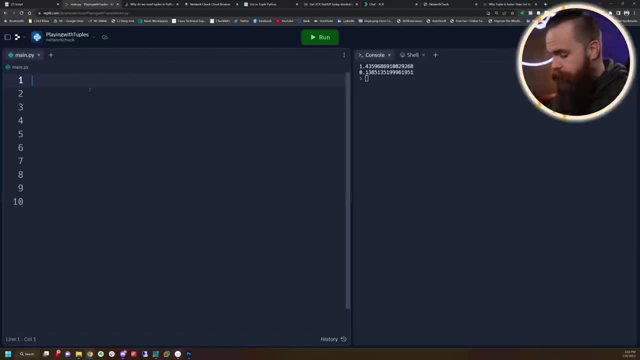 cool, You can unpack a tuple. So, for example, let's say we have this two point. I'll call it network Chuck, I'll hide it. equal my name, my age and my favorite drink, coffee. I can unpack this and assign it to multiple variables all at once. 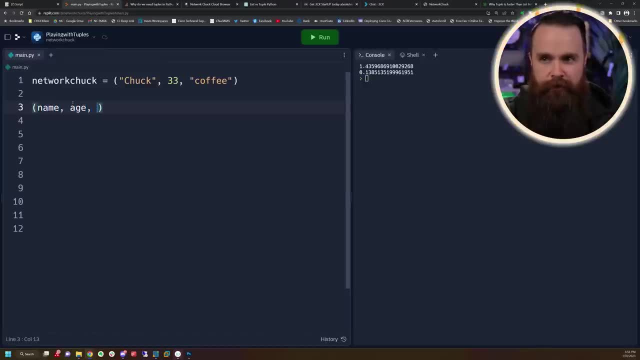 By doing this I'll create three variables: name, age, drink and half that equal the two pool network. Chuck And that legit made three separate variables that have packed it. As long as you have them in the correct order, they print all of them real quick: print name, print age and print drink. 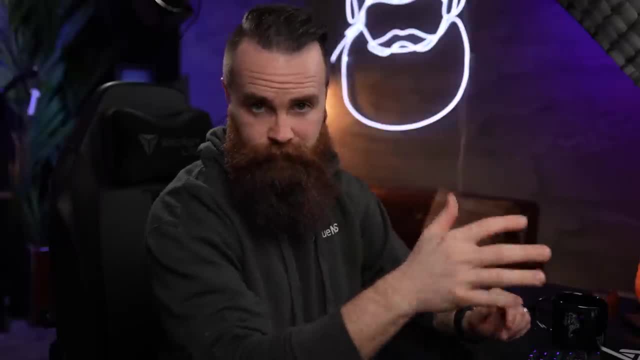 It's pretty cool, right, Which, by the way, you can do the same thing with list. So just now, you know it's not unique to two pools, but I hadn't talked about it yet. I wanted to show it to you now. Also, two pools are kind of weird. 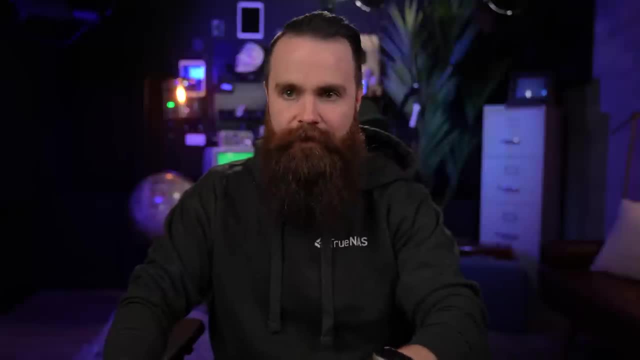 You probably saw this coming because they have a weird name. It's a two point. I don't even know how to say it right. Is it tuple or two pool? I don't know. Comment below: You probably don't know this. 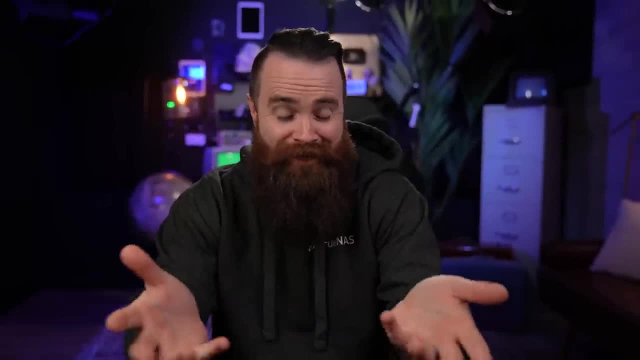 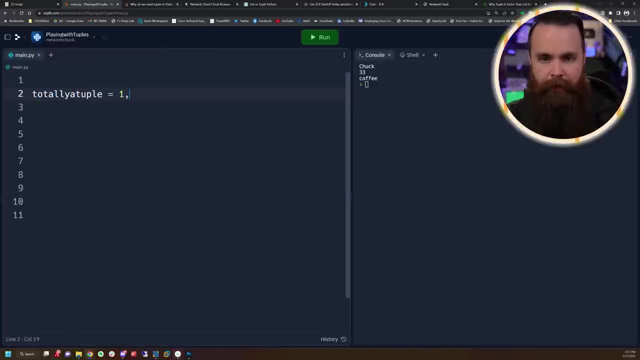 You don't actually need to use parentheses to make a two pool. Seriously, Watch this- totally a two pool, So I'm gonna name this thing equals one And then to make it a two, I don't need parentheses, All I have to do is just add a comma. I don't even need more than one piece of data. 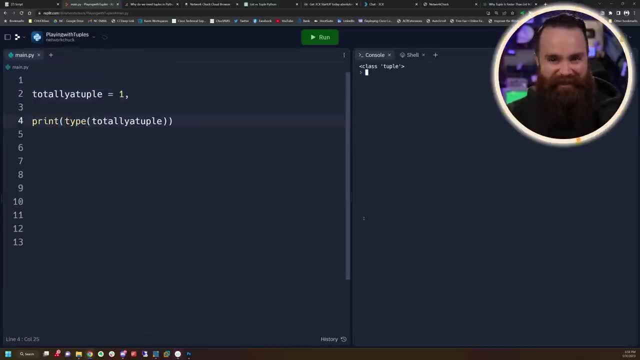 If I print to the type of that data, it's a two pool, which is so weird, So you actually need parentheses. All you need is a comma. Okay, I've got multiple pieces of data, psych. So, yeah, it's weird.